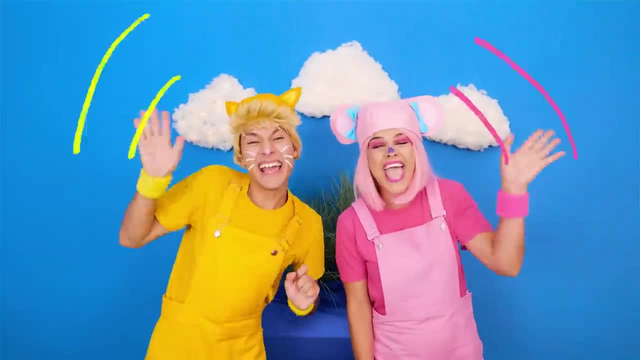 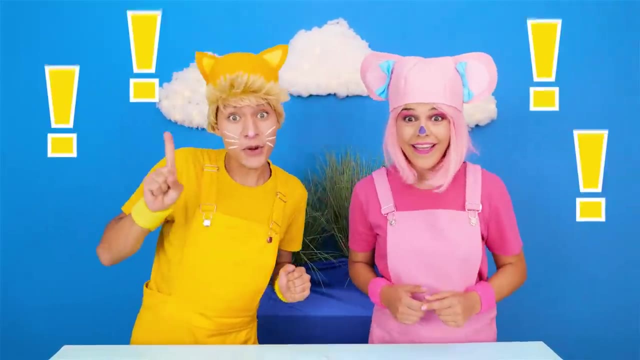 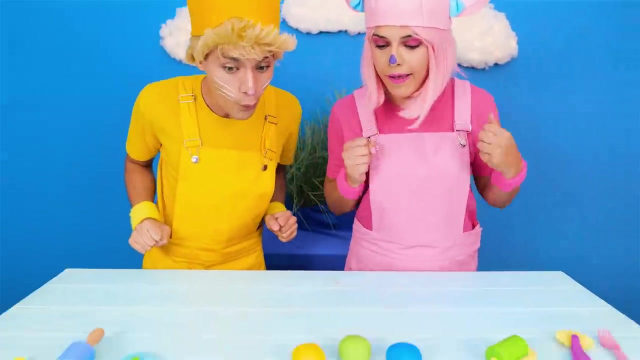 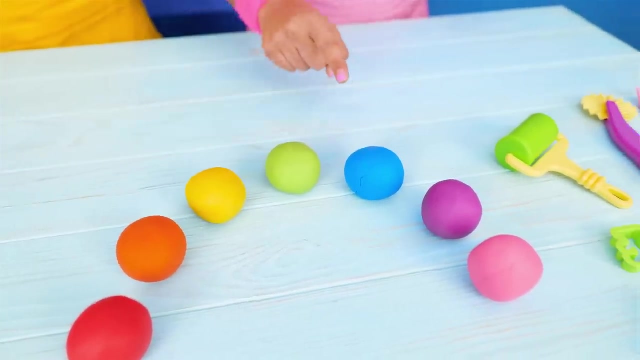 Peek-a-boo, Hello. Today we're going to play with clay. You can play too, But don't forget, always play with a grown-up beside. We've got so many colours. Look: Red, orange, yellow, green, blue, purple and pink. 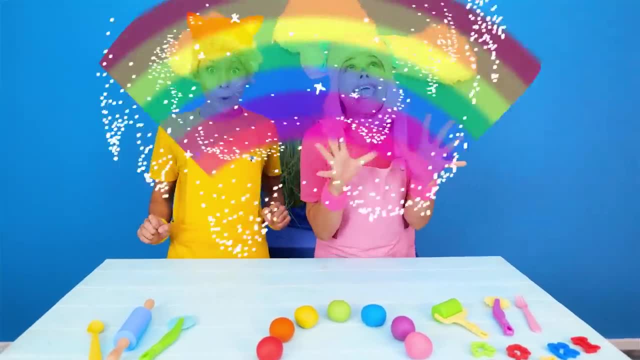 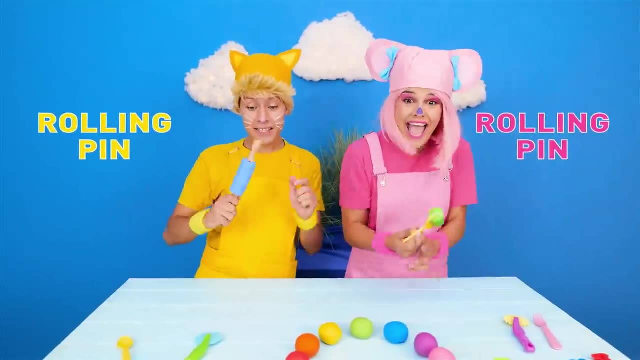 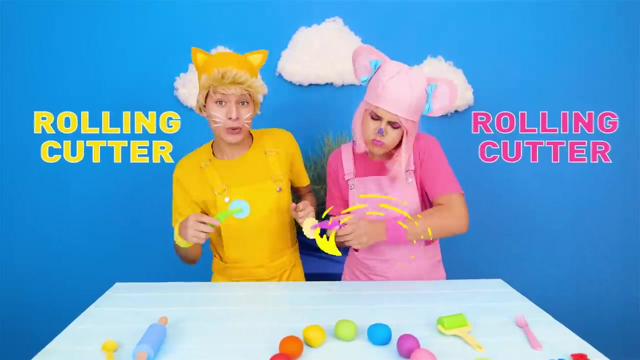 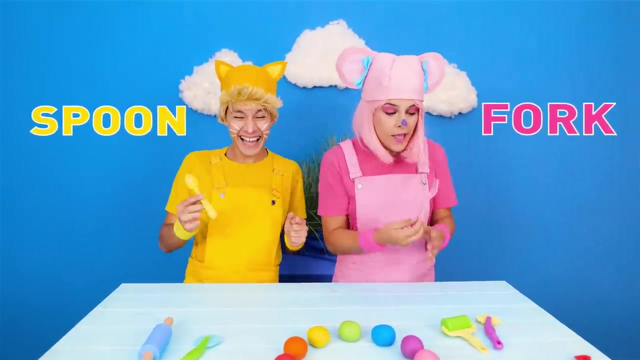 It looks like a rainbow And we have so many things to play with: A rolling pin to make the clay nice and flat, a rolling cutter to cut the clay in half, a spoon and a fork. Now we're going to find the cookie cutters. 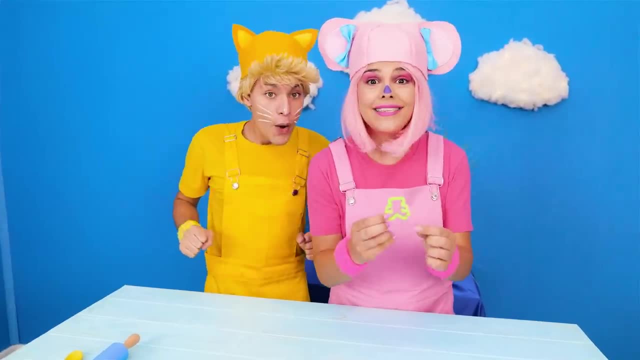 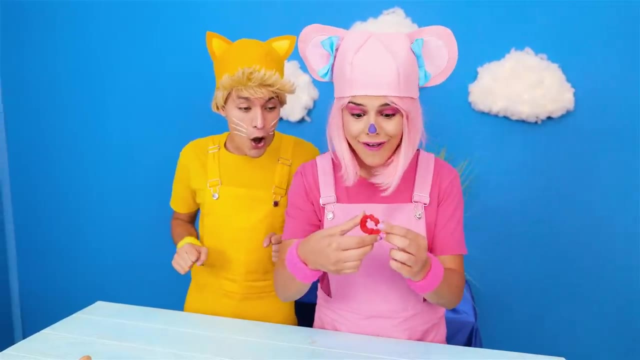 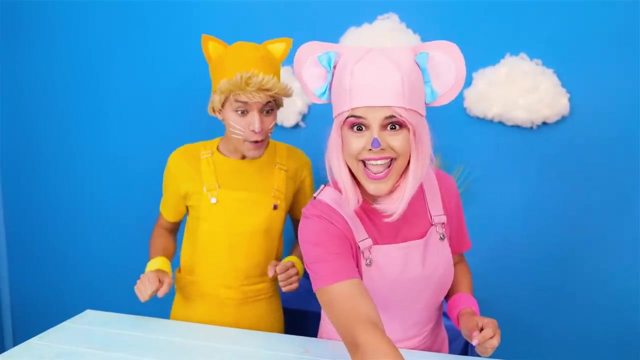 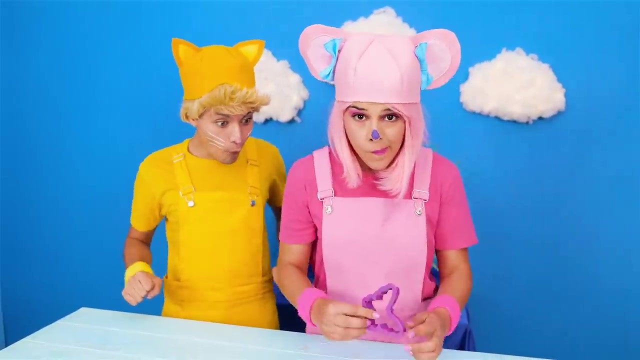 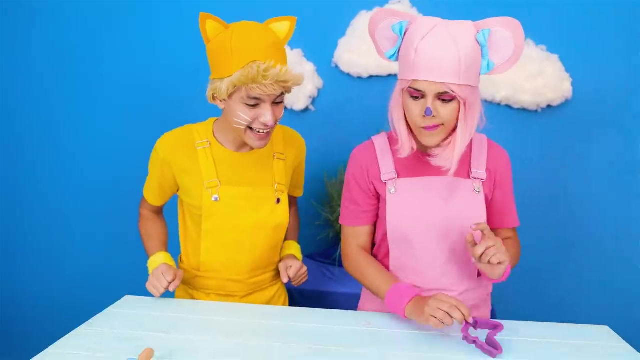 This is a cookie cutter. It's a nice teddy bear And look, I've got a tree And a twinkly star And a big, beautiful butterfly. I'm going to choose the butterfly. Now let's pick a colour. 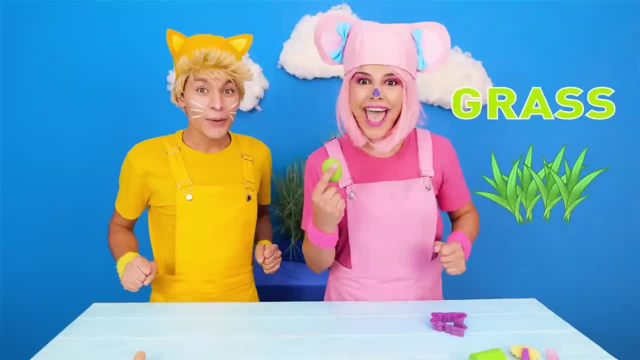 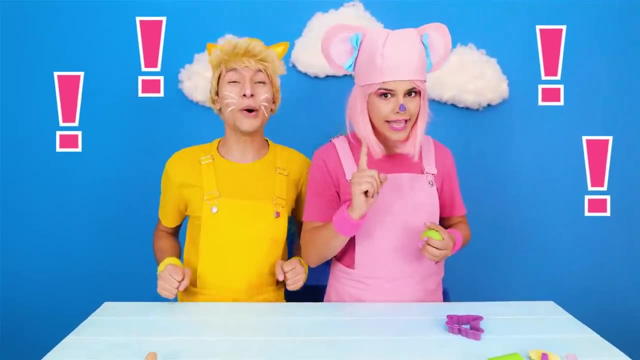 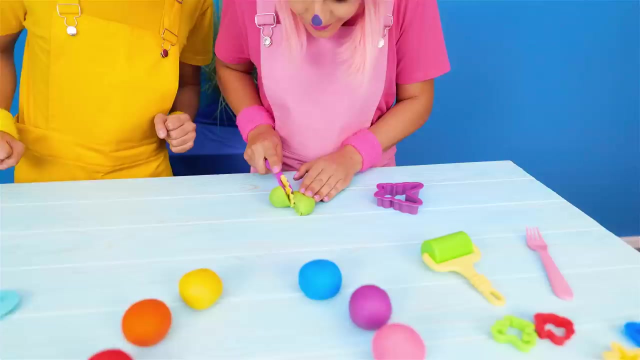 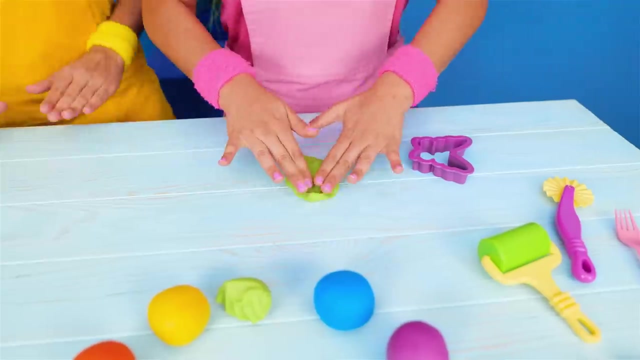 I'm going to choose green. Green like grass, Or like green apples. Oh, don't eat it. We don't eat clay. We play with clay. We're going to cut it in half, Squish it, Make it flat. 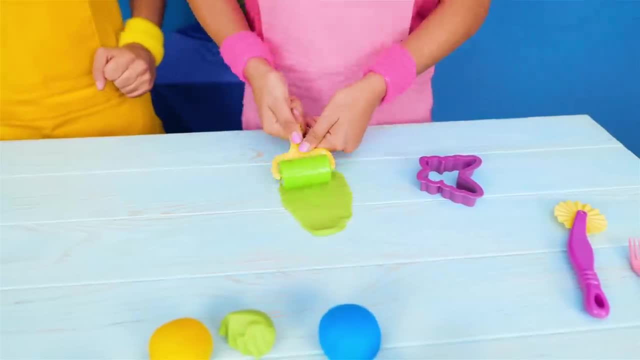 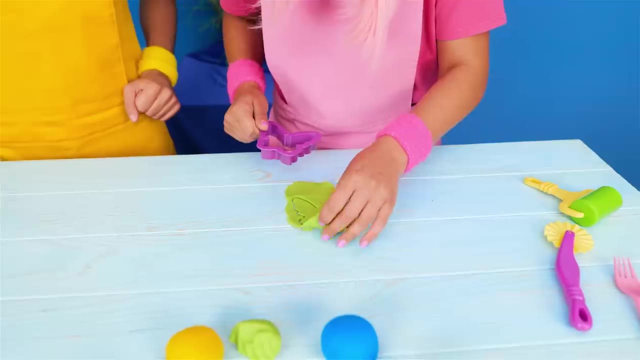 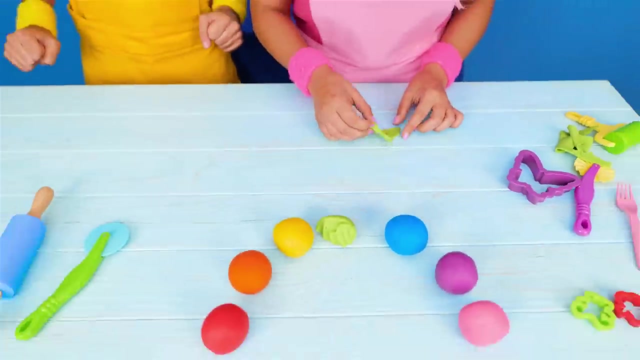 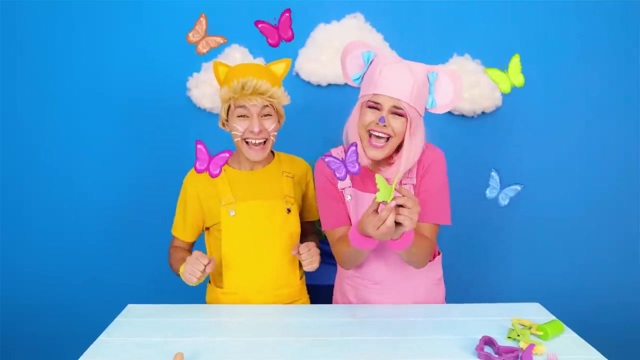 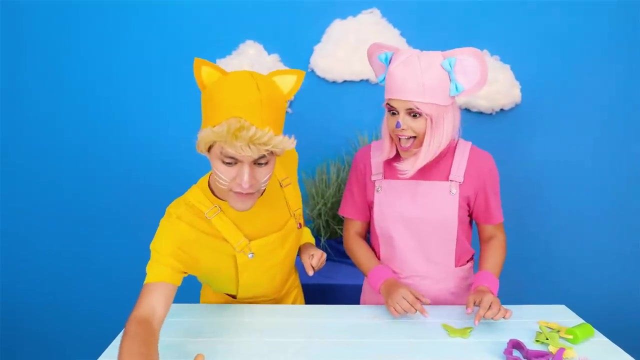 Oh, wow, This is so cool. And now, Wow, A beautiful butterfly Fly, fly, sleepy, deep love. Do you like my butterfly? I want to do something too. Let's see, I have A tiny elephant. 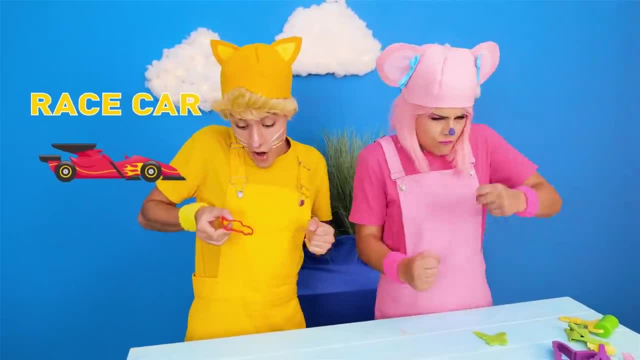 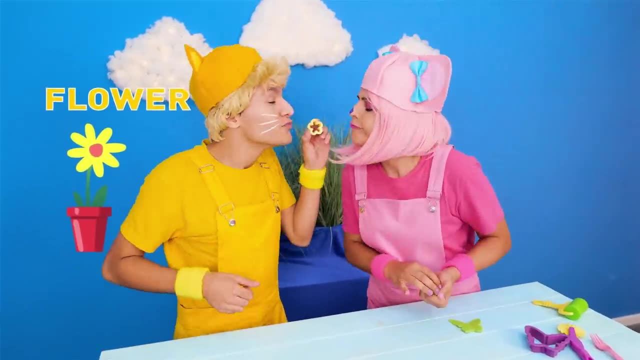 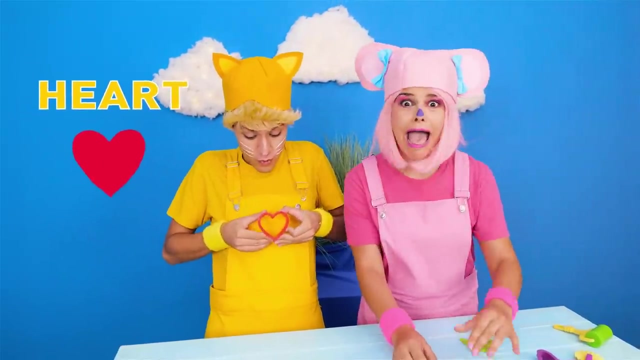 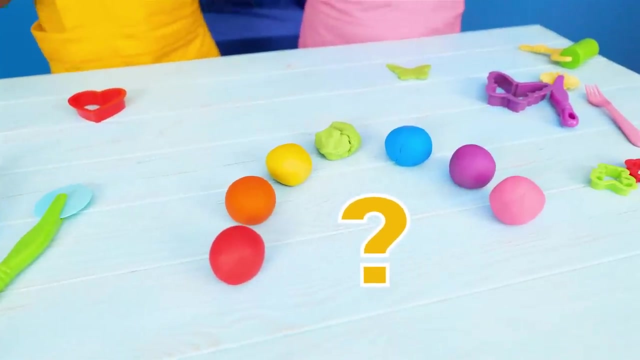 Whoa, A race car, A beautiful flower And a big red heart. Oh wow, I'm going to use the heart And I want to make it Blue. That's a nice colour. It's like a big, beautiful sky. 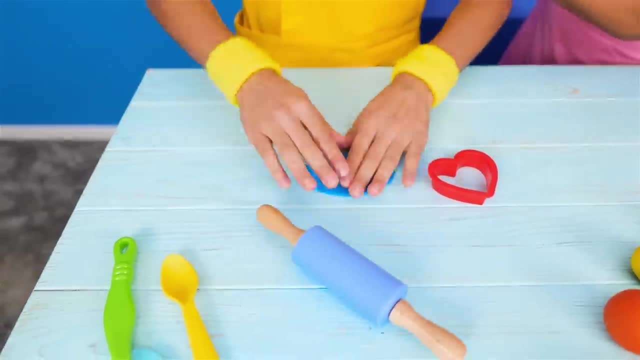 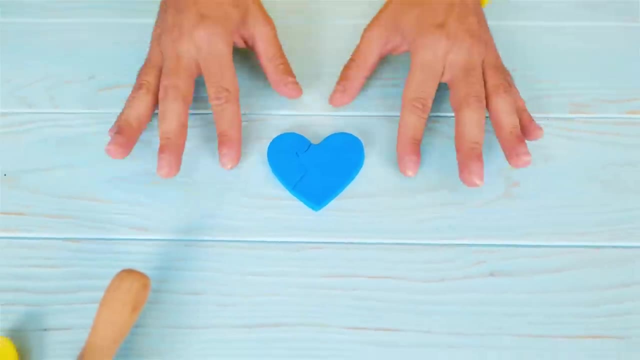 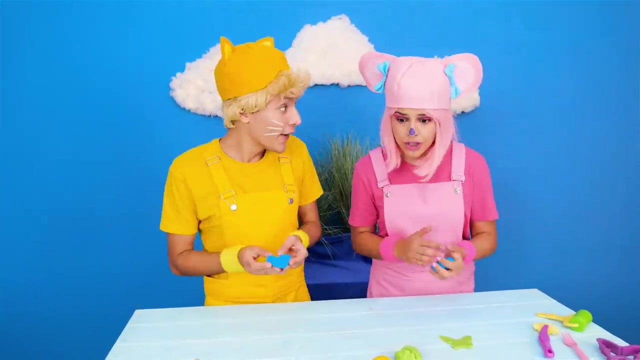 Oh, look at that. Wow, Such a beautiful blue heart. I know what else we should do today. Do you know what my name is? I know what your name is. What is it? It's Kiki Yay. 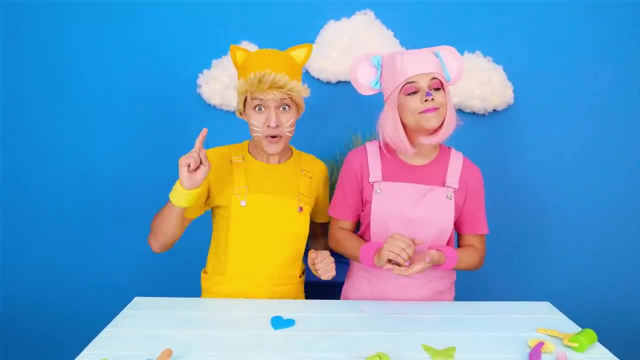 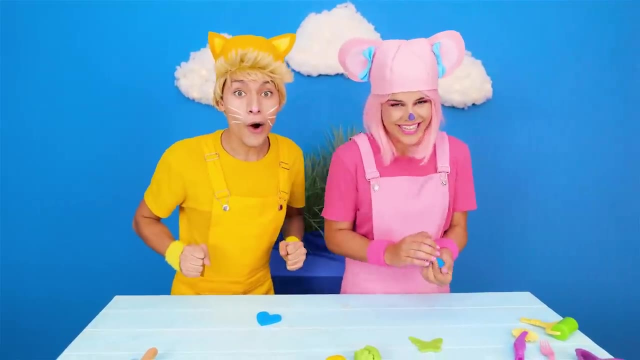 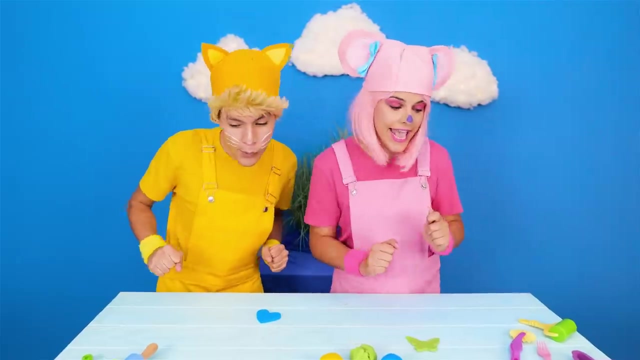 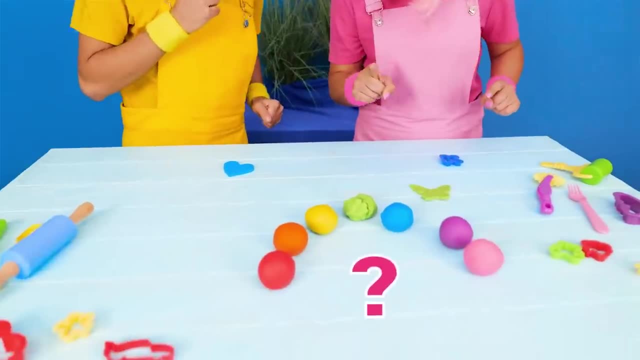 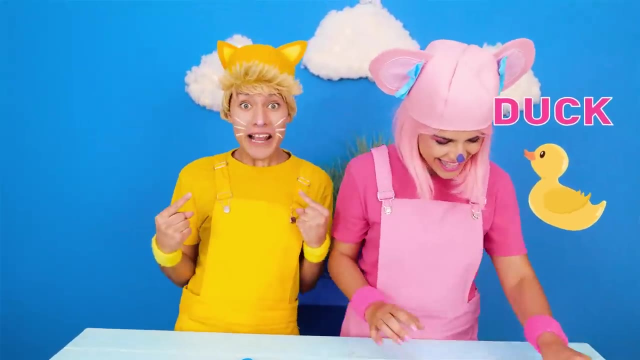 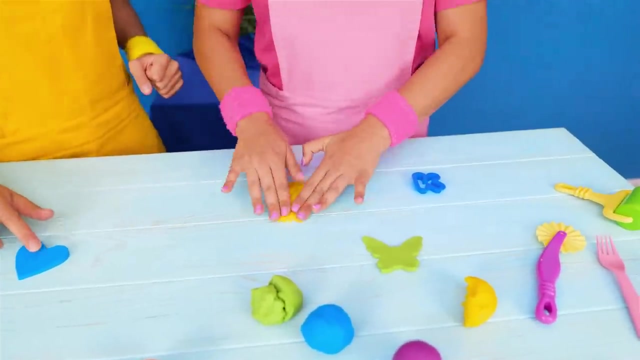 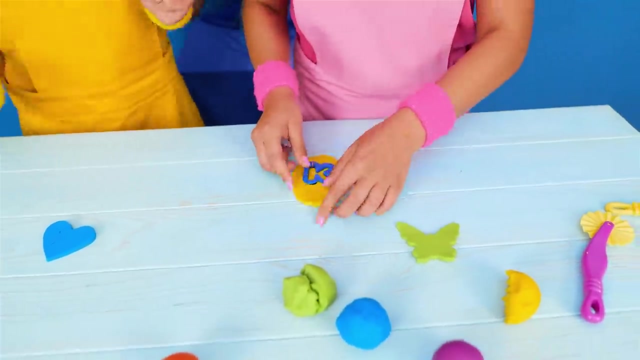 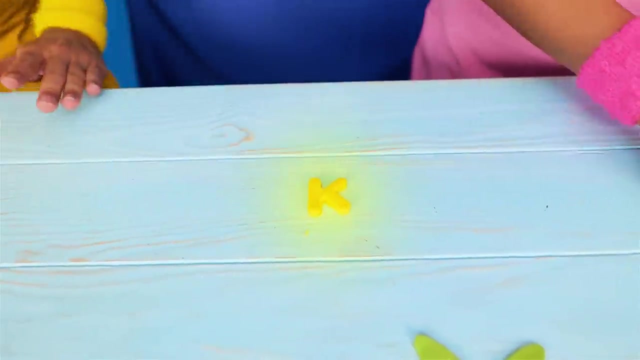 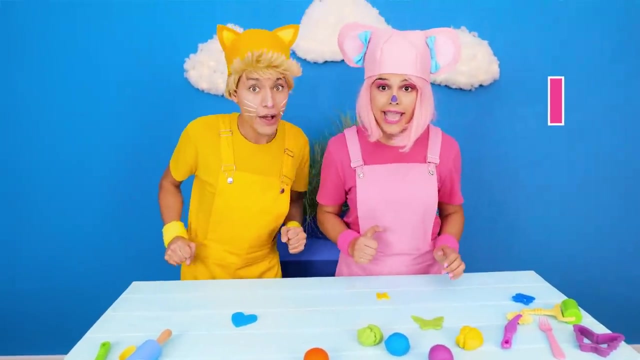 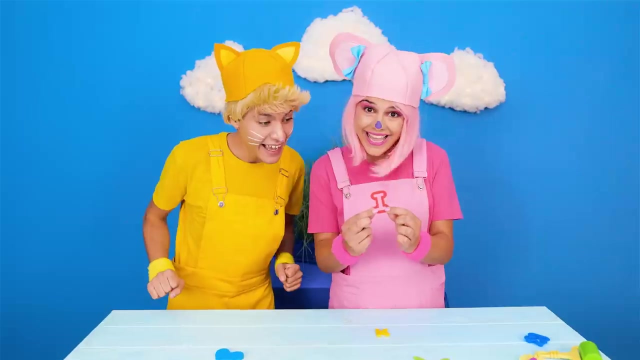 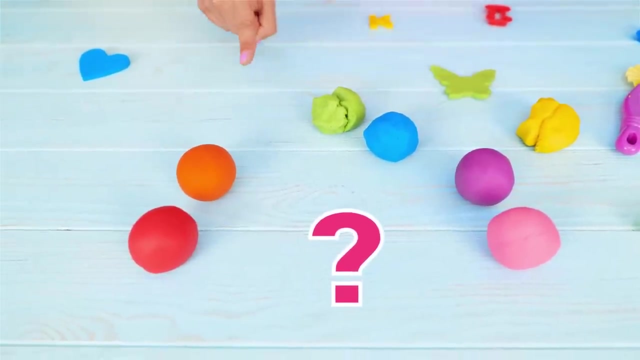 Now let's pick a colour: Yellow, Yellow Like duck, Or like me. Yay, Whoa, it looks so good. Now we need: I, I like, I am I. hmm, let's pick a color. hmm, red, red like a rose. 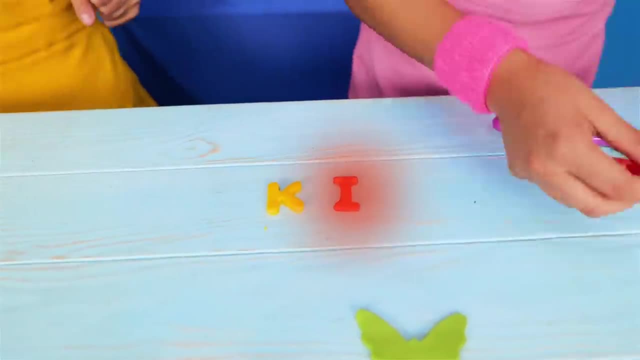 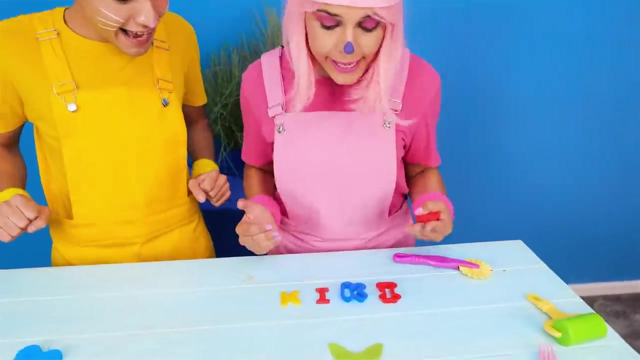 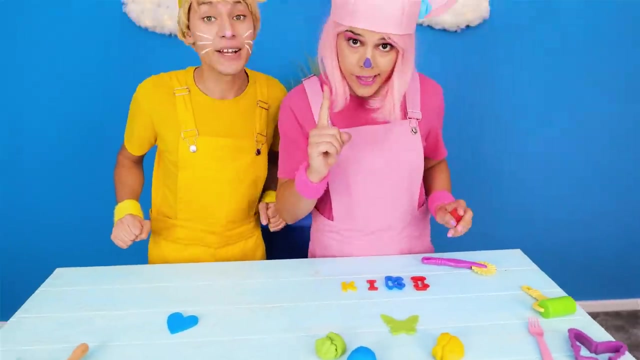 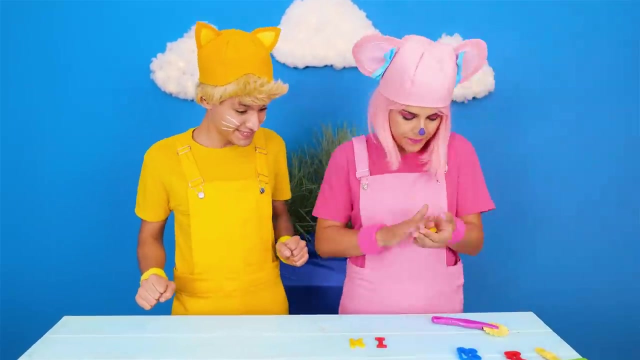 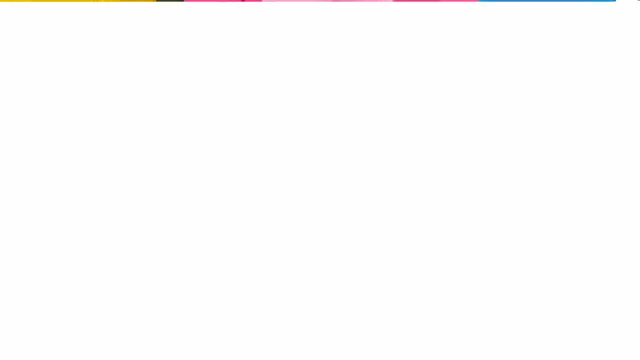 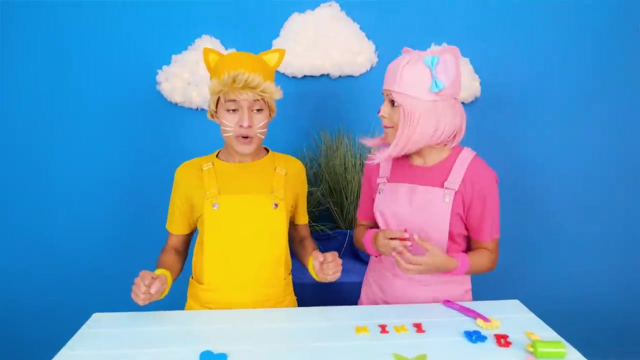 It looks so good. Now we need one more K and one more I, and you will be Kiki. I'm going to use the same colors and the same letters: K with yellow. I want to do something too, but I'm going to make my favorite animal the panda. 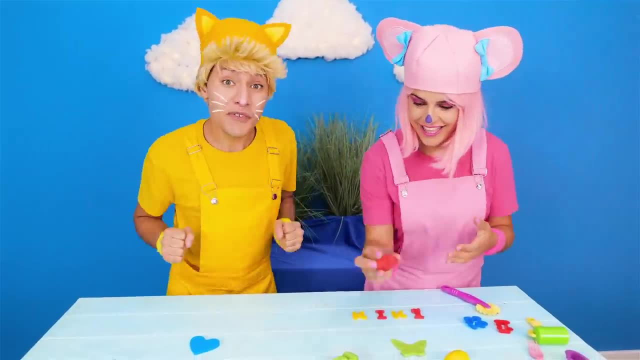 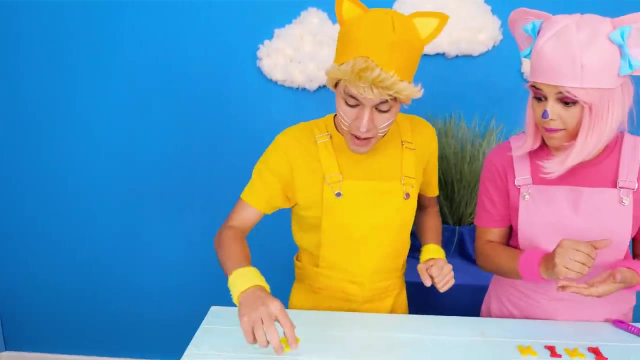 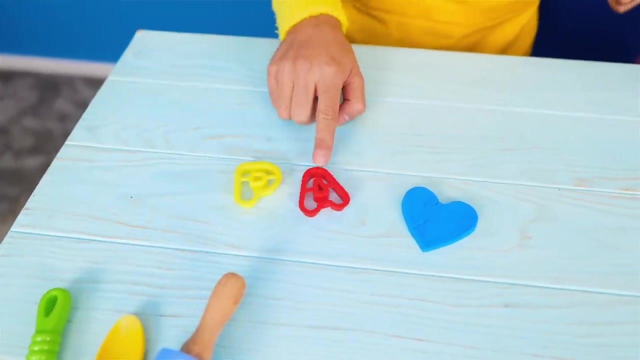 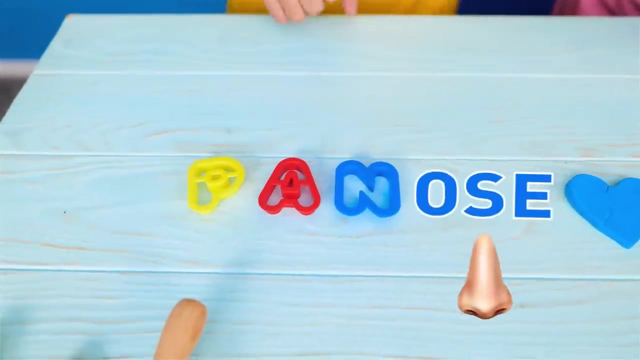 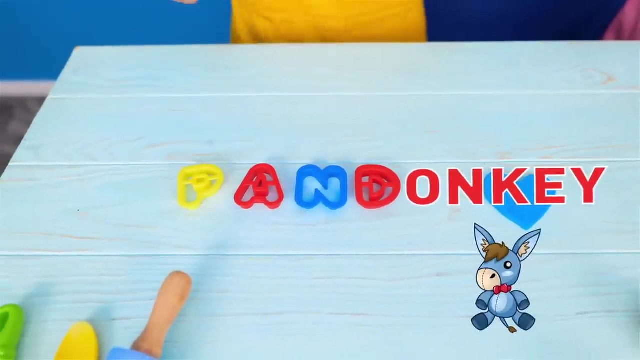 So cute and fluffy. What's your favorite animal? Okay, All right, For panda. we need P like panda, Yeah A like an airplane, N like nose, yeah D like a donkey, ee-ah, ee-ah. and we need 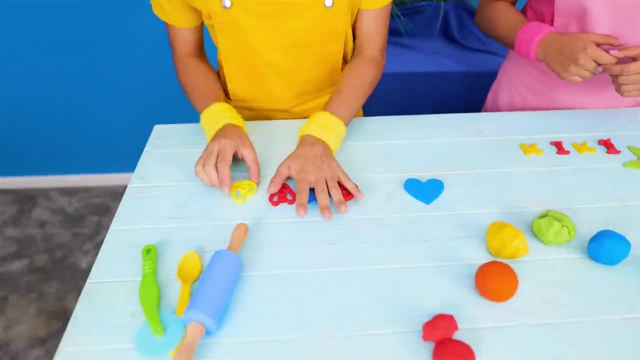 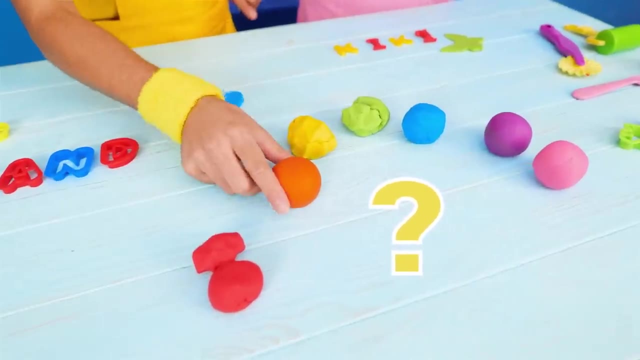 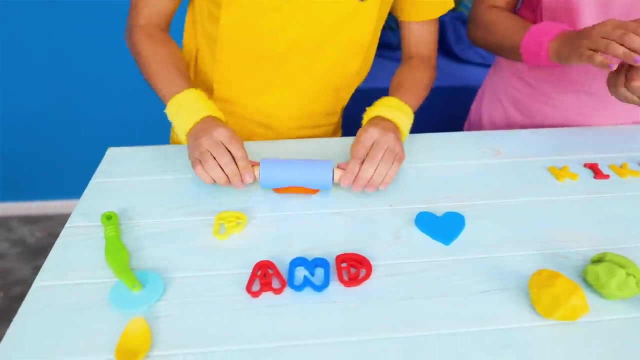 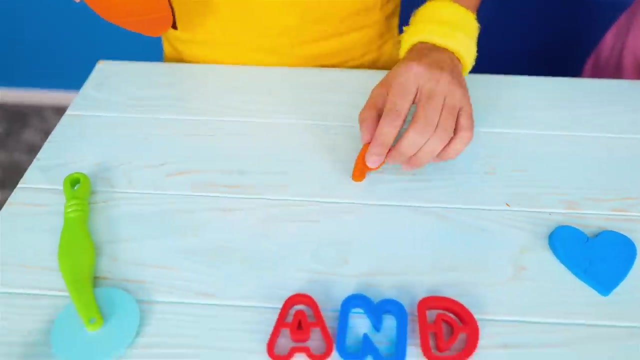 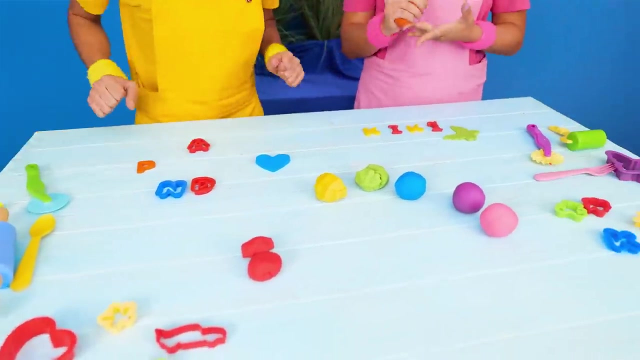 A again. All right, Let's start with the P. I'm going to make it. I'm going to put orange. ooh, like an orange. It looks amazing. All right, Now the A I'm going to use. I want to use green too. 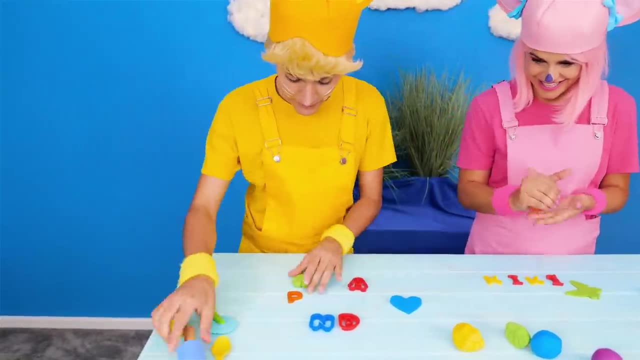 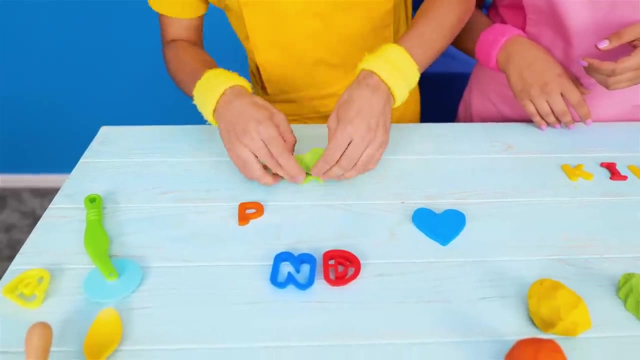 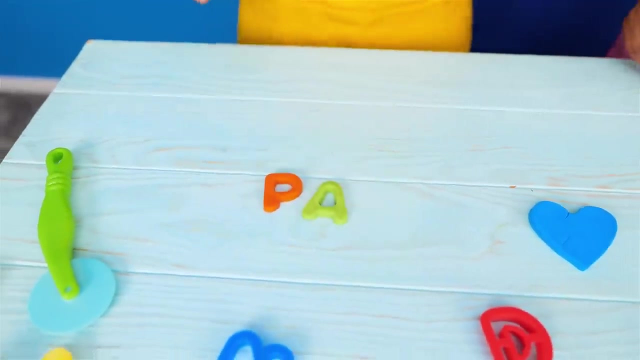 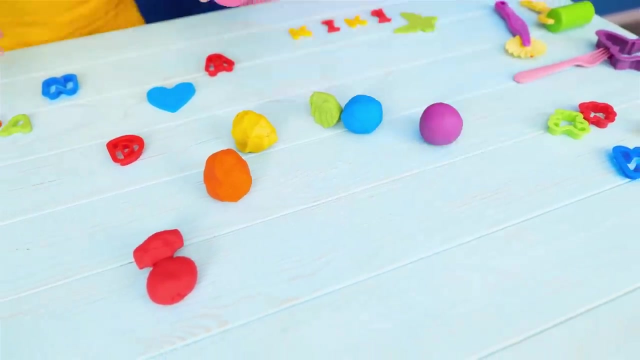 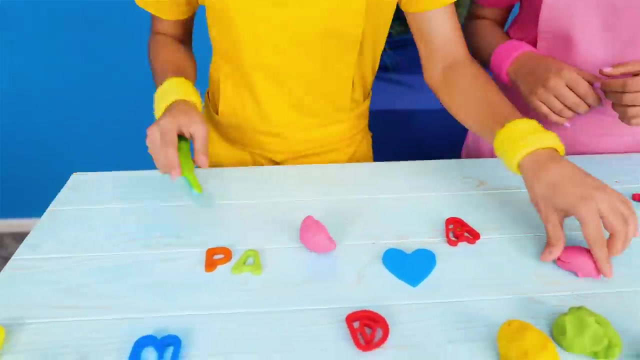 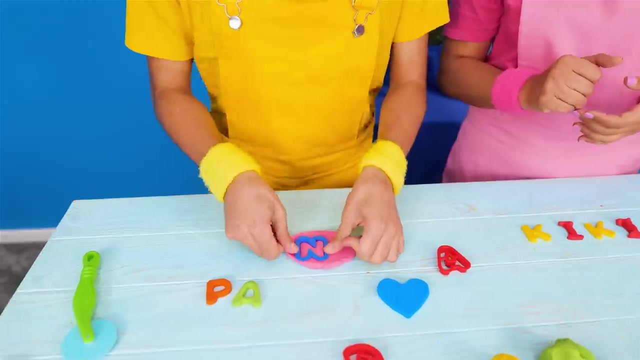 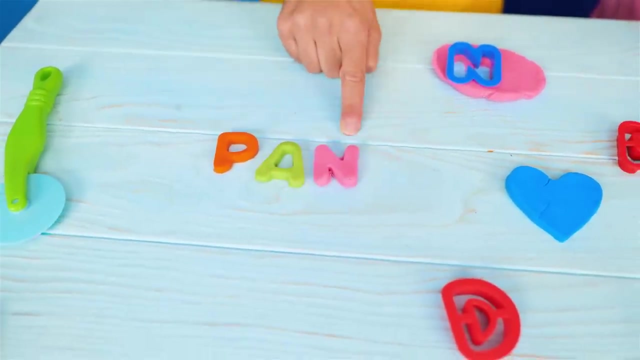 Whoa, I'm going to use pink. All right, Here we go. A. Now we need N, and I'm going to make it pink, like me. yeah, just like you. Yeah, I got it. And P. oh, we're still missing letters.